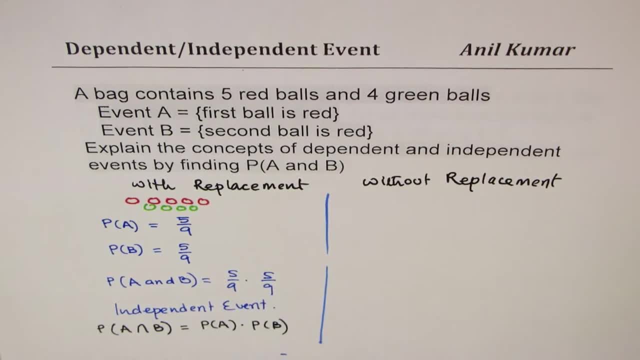 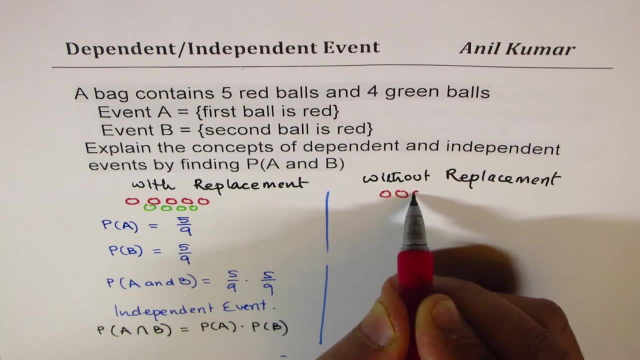 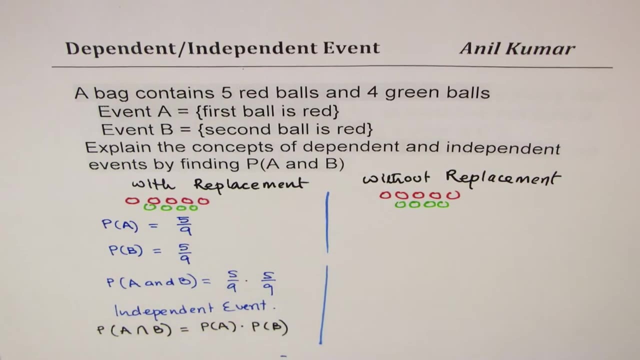 times probability of B. right Now, if we take the second case where we again have five red balls and for green balls now if we consider the case without replacement, in that case probaminebt of picking the first red ball is five out of nine, five red out of total of nine. so now if we take the 2nd case where the ellisp thinker has recognised at the 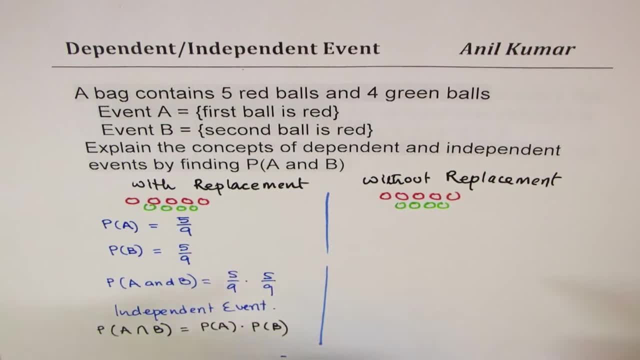 case without replacement. in that case, probability of picking the first red ball is five out of nine. five red out of total of nine. we have a boxought match watch now, thereforeE out of 9, right, 5 red out of total of 9 balls. Now the second red ball, that is, if we put 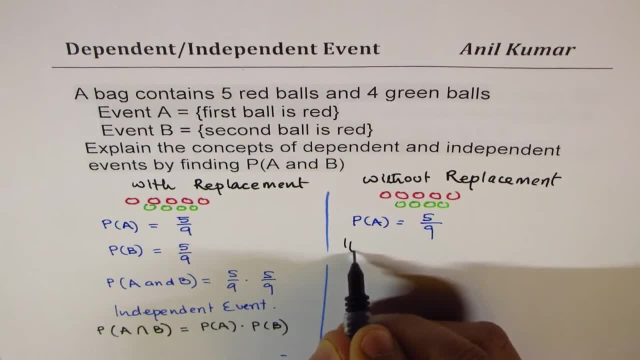 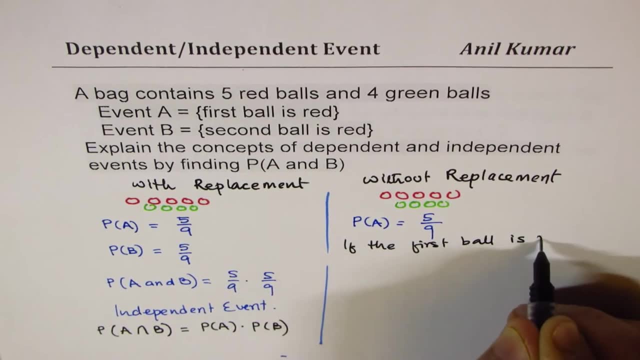 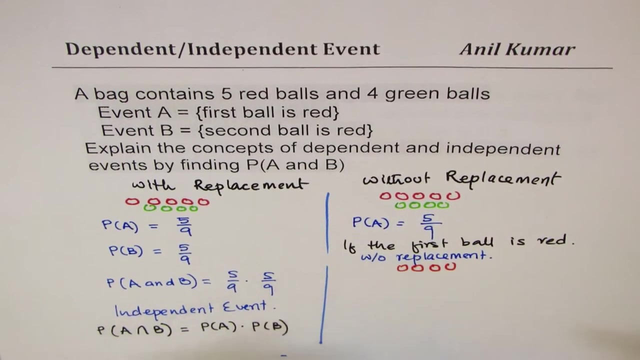 a condition here, that if the first ball is red, in that case what happens? And we are not replacing, right? We are talking about without replacement, So just the conditional probability, right? So we are not replacing, we are left with just 4 red balls and 4 green. 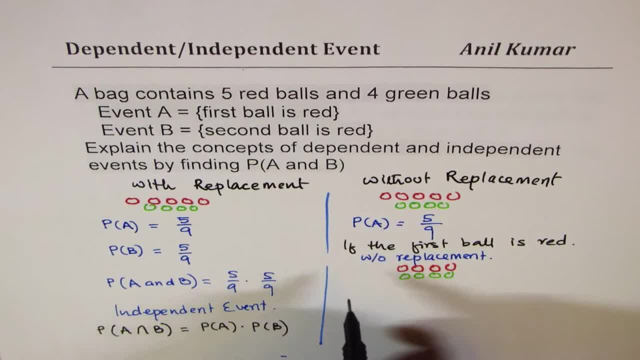 balls. So in that case we are talking about probability of event B when it's X or Y is equal to 0.. has occurred. do you see that probability of B, that is, the second ball, is red when a has occurred. so that means probability. 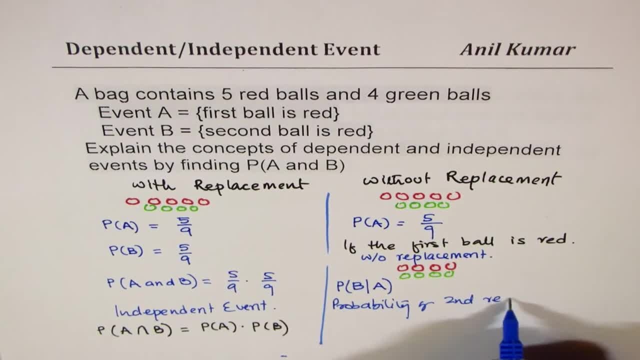 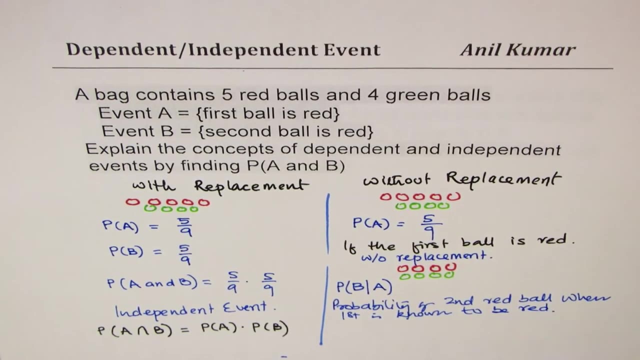 of second red ball when first is known to be read right. so that probability, since we know first is read, we are only left with four and there are total eight balls. so this probability is 4 over 8. so in this particular case, what you notice is that 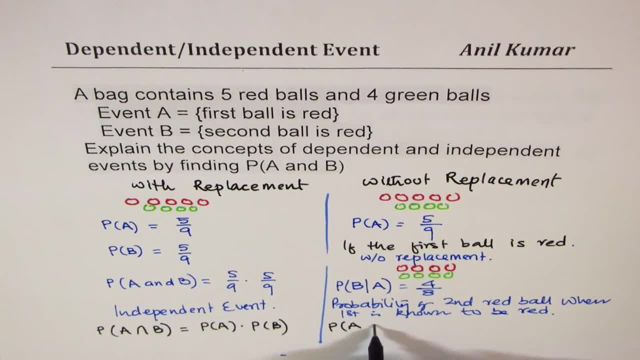 probability of A and B both to happen. that means two red balls is their product, which is probability of A times probability of B, when A has happened right. So in this case it is five out of nine times. this is half right times half product of these two. So that is how we get probability for 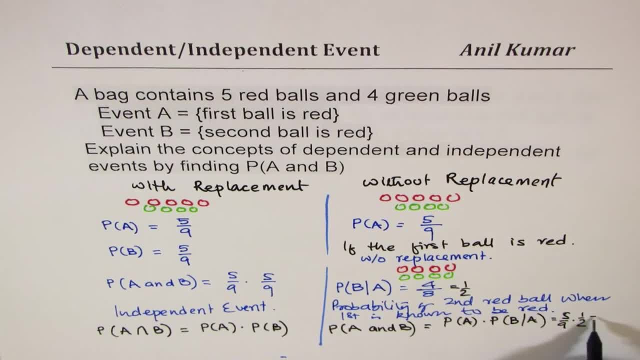 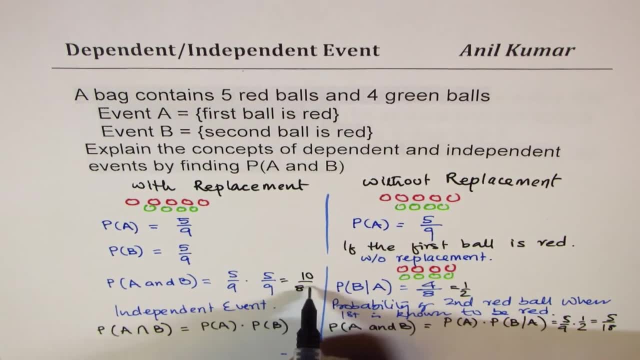 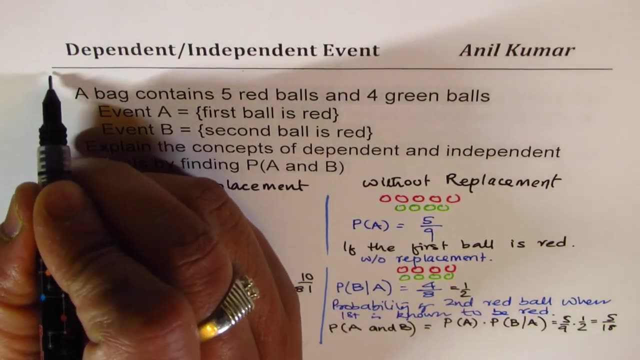 a dependent event, right So, which is 5 over 18, right So? and in this case it was 10 over 81.. So what you notice here is that in case of independent events, for independent events it is 5 over 18.. So in this case, it is 5 over 18.. So in this case, it is 5 over 18.. 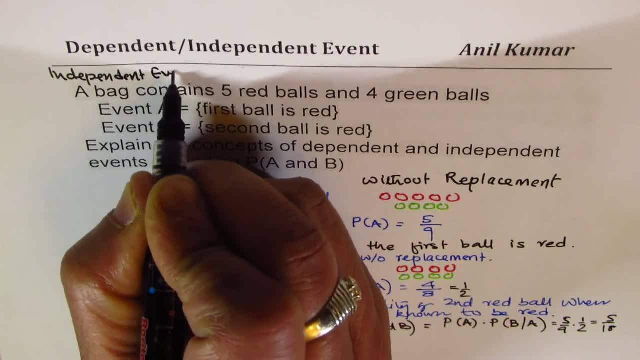 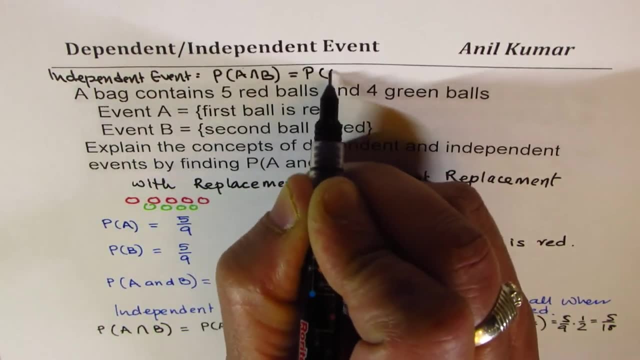 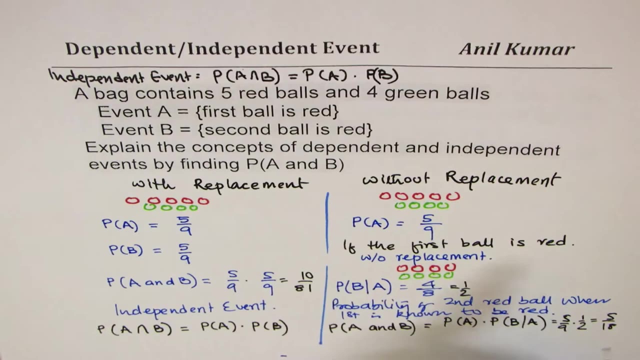 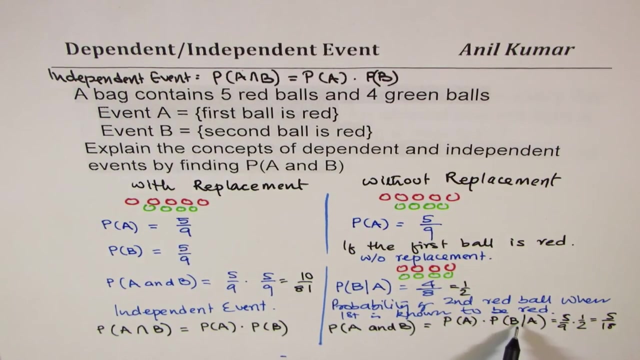 event, probability of a intersection B is equal to product of our probability of a and B. however, for dependent events, it is product of probability of a and the conditional probability of B happening when a has already occurred. right, so? so that is a huge difference. this is how we can summarize the two differences, so I 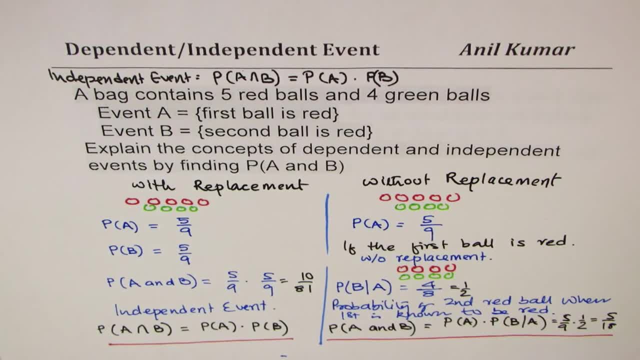 hope with this video, the concept is absolutely clear. so in independent events, probability of both the events to occur is the product of their individual properties, and for a dependent event, you probability for both the events to occur is product of probability of a times probability of B when a has occurred. right, so that is how we could actually 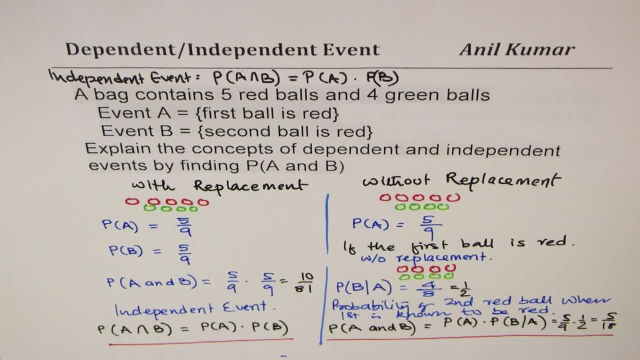 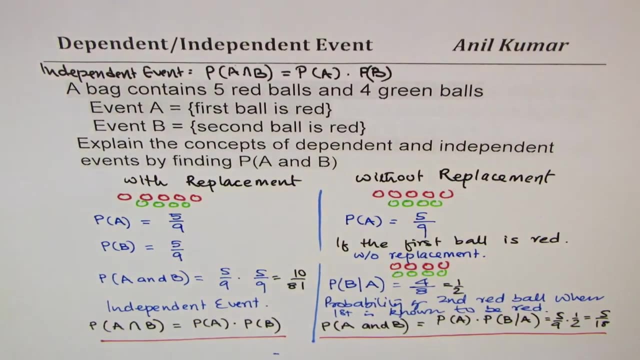 distinguish between them and understand the concept of dependent and independent events. I hope that helps. feel free to write your comments and share your views and, if you like, and subscribe my videos, that'd be great. thank you and all the best you.